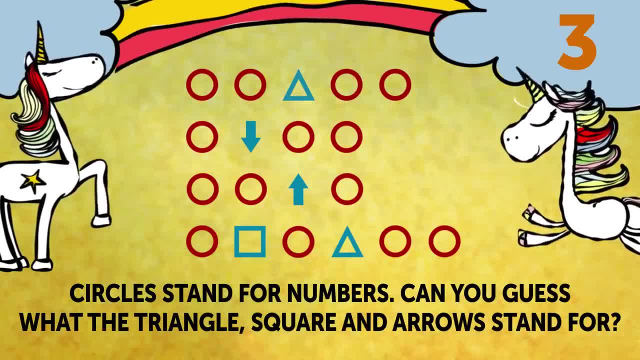 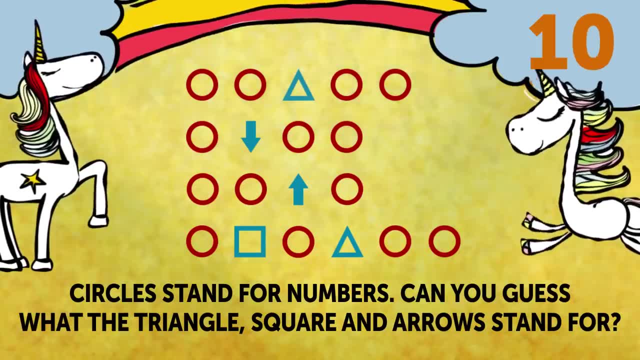 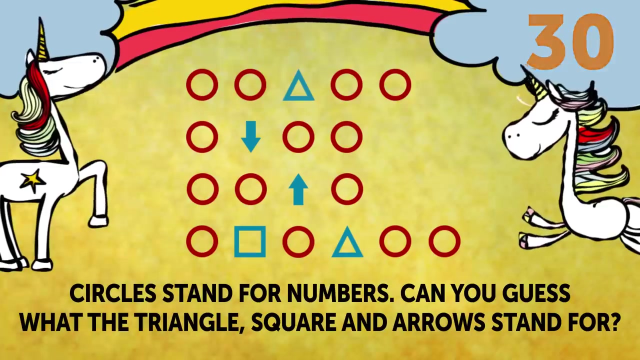 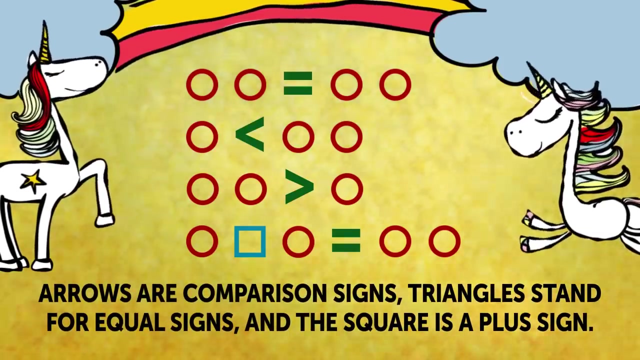 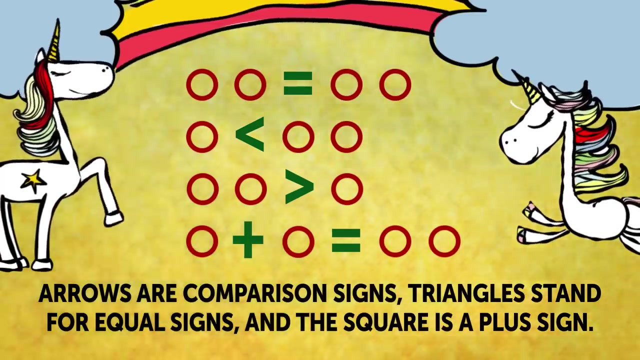 You'll have 30 seconds for this tricky puzzle. That was a good one, And here is the explanation: Arrows are comparison signs, Triangles stand for equal signs and the square is a plus sign. It all makes sense now, 4.. 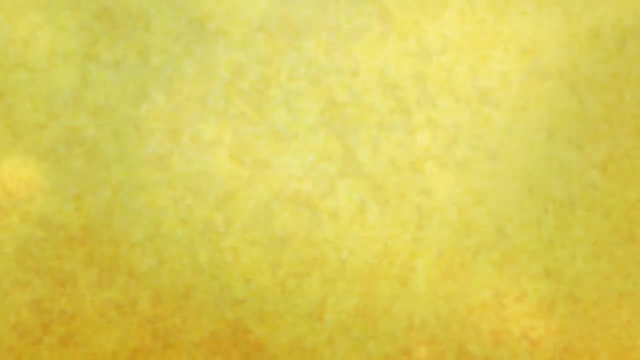 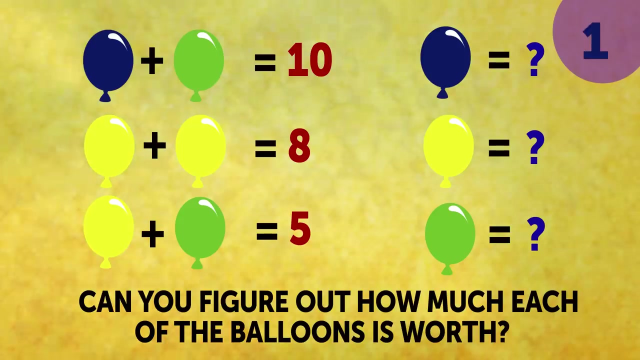 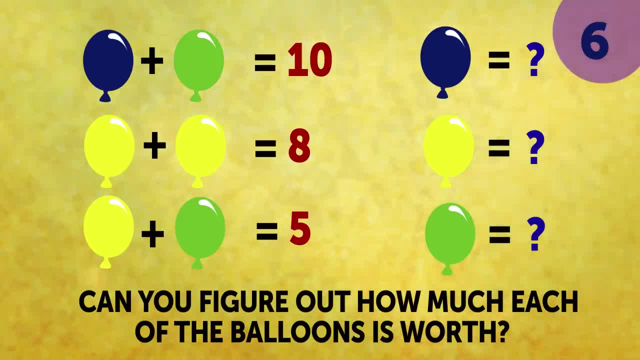 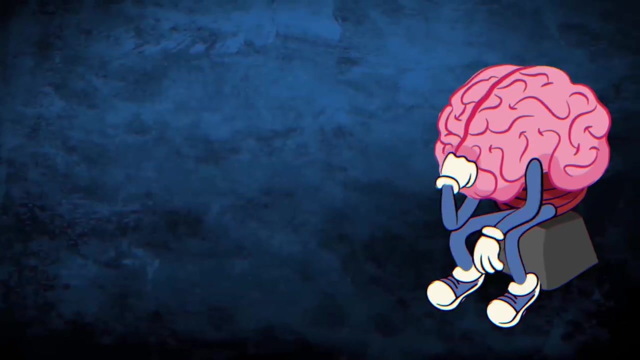 The answer is 6.. 5. Theину equation. That was easy, wasn't it? The blue balloon is a 9,, the yellow balloon is a 4, and the green one is a 1. Number 5. Flower equation. 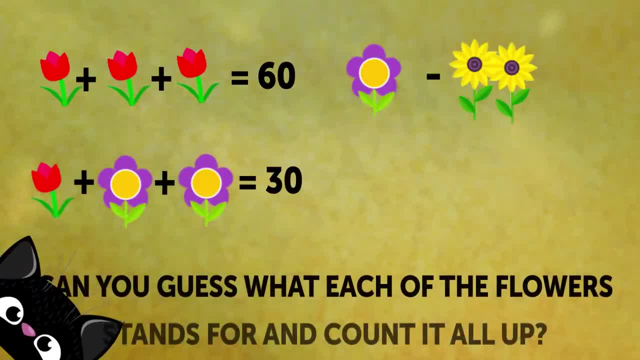 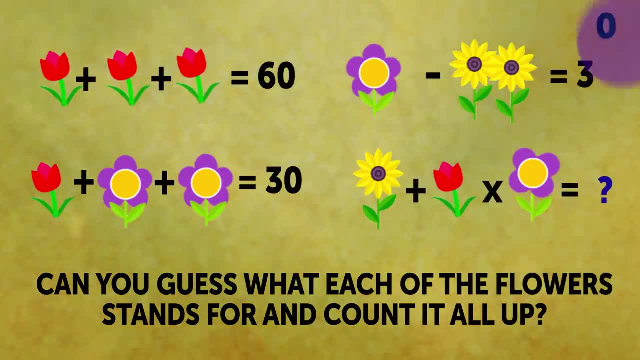 Another fun equation. that looks like spring. Can you guess what each of the flowers stands for and count it all up? Your 30 seconds for the task start now. Well, before I give you the final answer, let's go along each line. 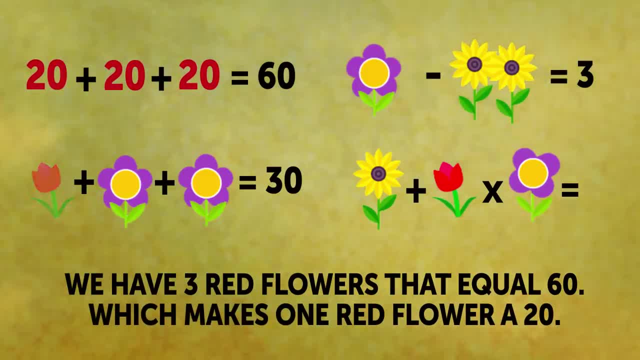 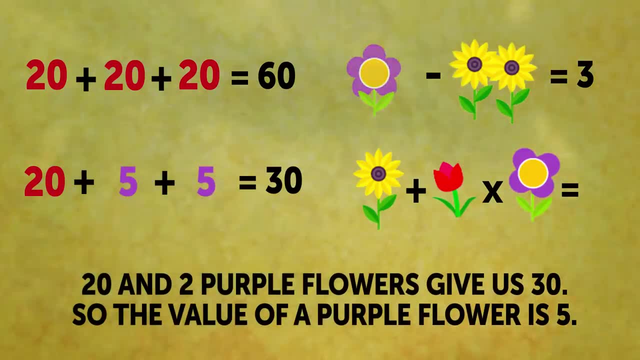 We have 3 red flowers. that equals 60, which makes 1 red flower a 20.. 20 and 2 purple flowers gives us 30,. so the value of a purple flower is 5.. 5 minus 2 yellow flowers equals 3.. 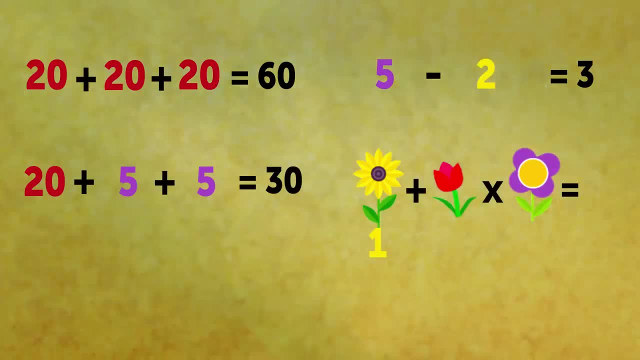 So now I see that a yellow flower is a 1.. Finally, let's go along each line. Let's go along each line. Let's go along each line. Finally, 1 plus 20 times 4 gives us 81.. 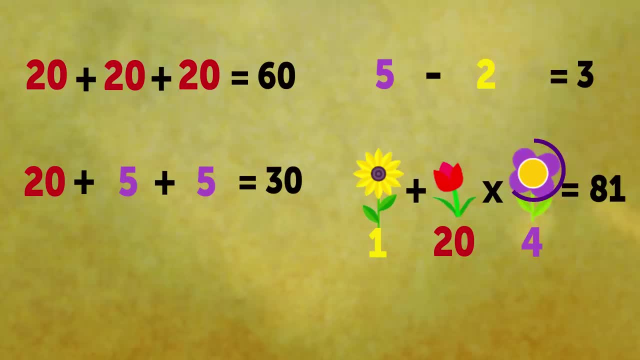 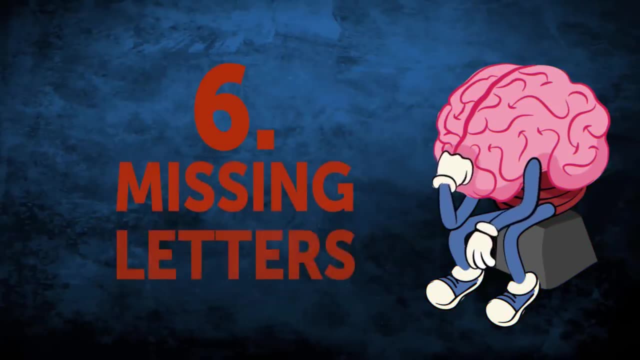 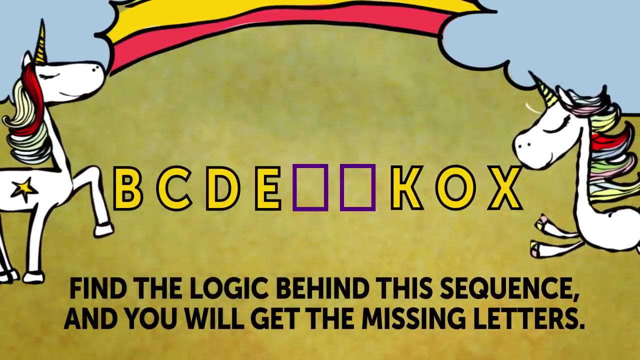 Why do we multiply by 4 and not 5?? Because the flower is missing one petal: Number 6.. Missing letters. Find the logic behind this sequence and you will get the missing letters. Give it some thought. You've got 30 seconds. 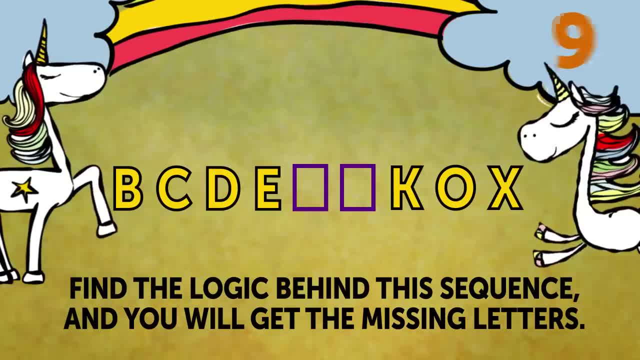 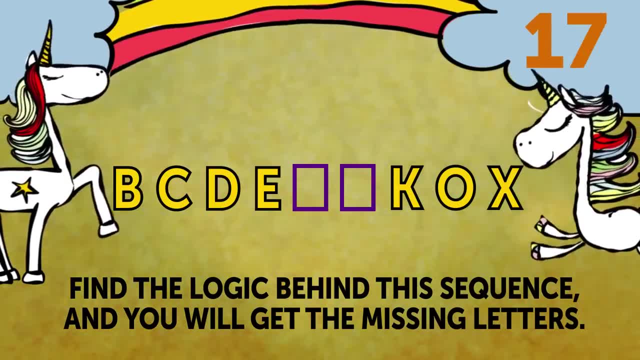 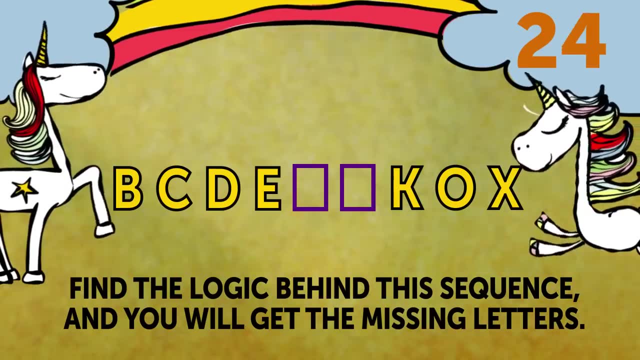 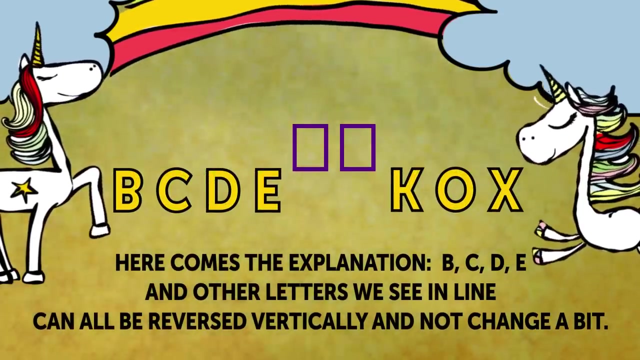 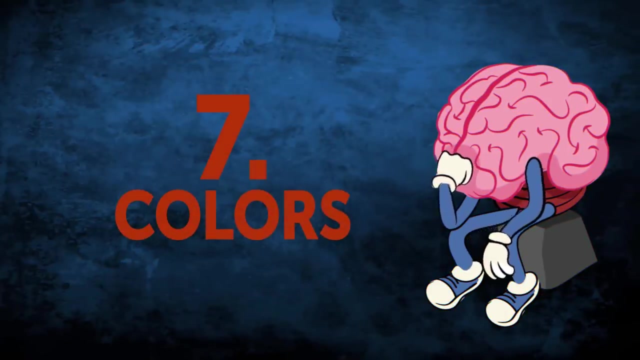 Here comes the explanation. B, C, D, E and other letters we see in line can all be reversed vertically and not change a bit. Following this logic, we can add H and I to the list Number seven Colors. You should figure out which number. 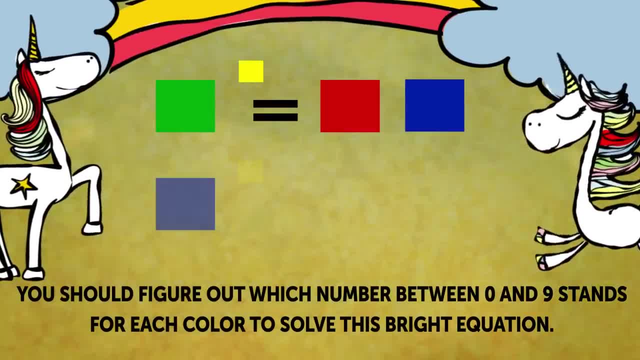 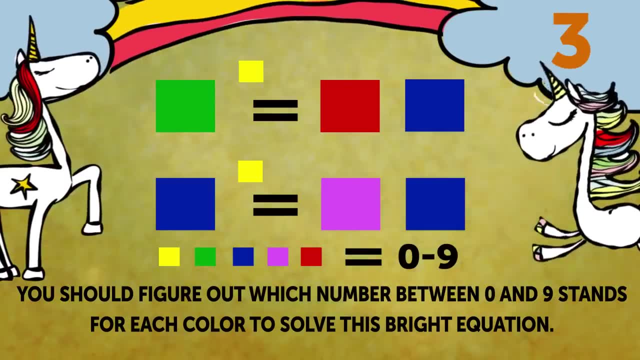 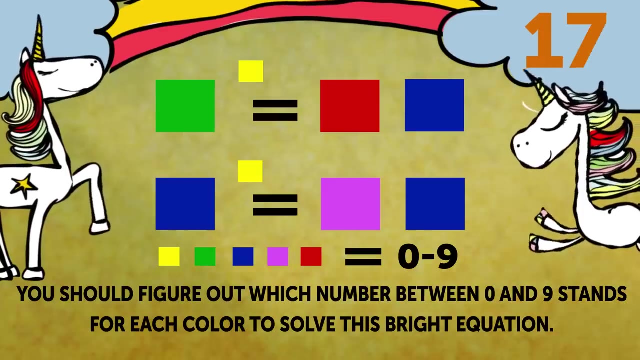 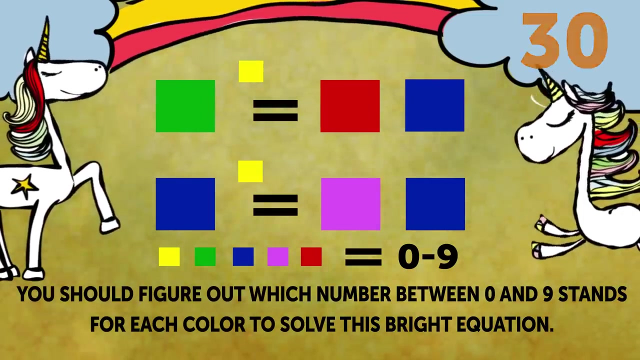 between 0 and 9 stands for each color. to solve this bright equation Take your time, but no longer than 30 seconds. 10 seconds to go Time to check out the answer. 4 squared equals 16.. 6 squared is 36.. 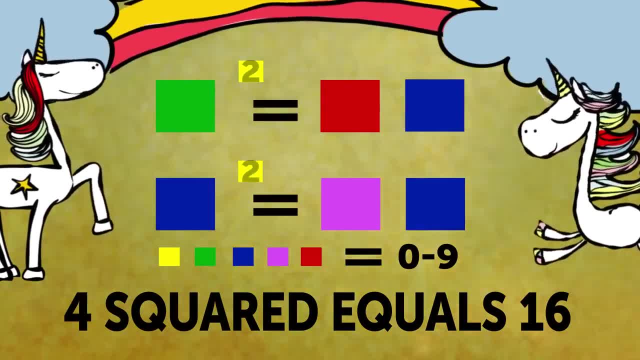 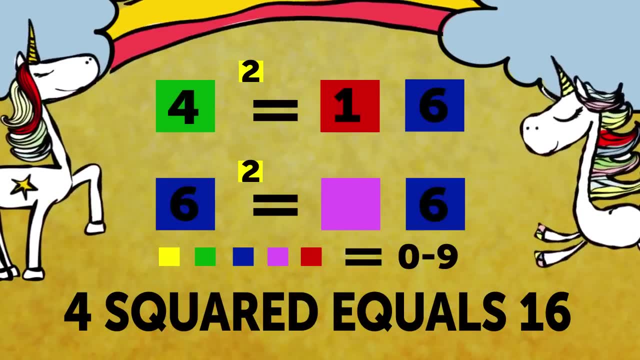 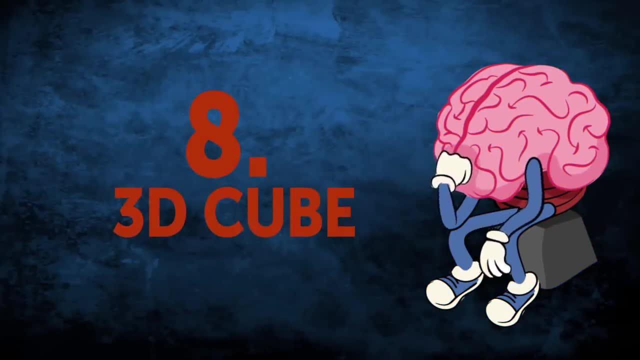 So here are the numbers for each color: Yellow is 2., Green is 4., Blue is 6., Red is 1. And pink is 3.. Number eight: 3D cube. It's time to test your 3D visualization skills.